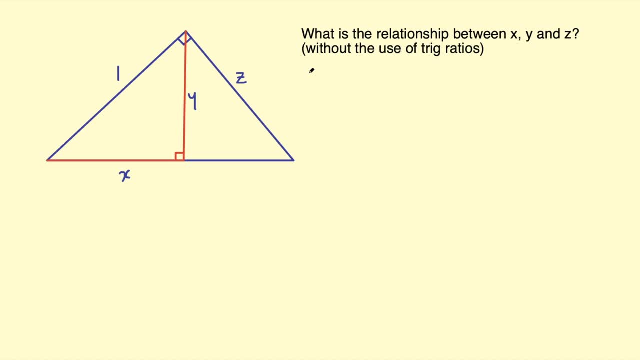 In this video I'll be talking about a geometrical understanding of the trigonometric functions and I'll briefly talk about where the names of sine, cosine and tangent come from. To show this geometrical understanding, I'll be using these two right angle triangles here, and I've written here: 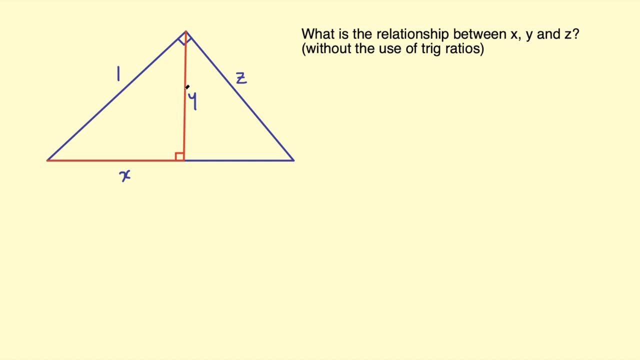 what is the relationship between x, y and z? so these lengths. and I don't want to use the trig ratios because I want to show that relationship, so I don't want to use them in my proof. So, looking at these two right angle triangles, what do you notice? Maybe pause the video here and write a few. 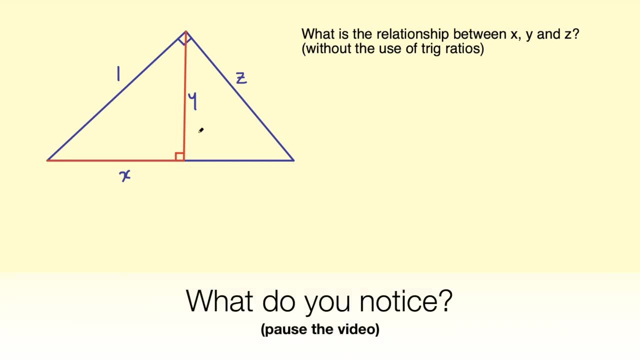 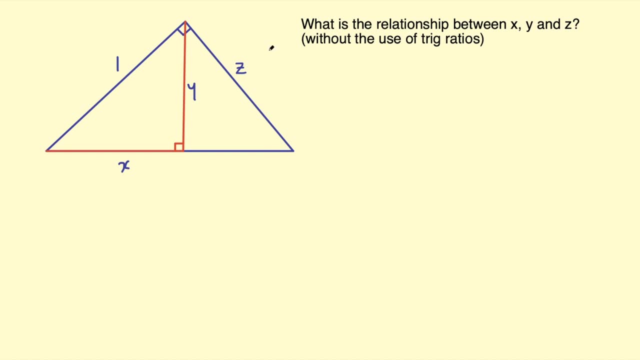 things down. The main thing is, and really the key to this relationship, is that these two right angle triangles are similar and we can show that using the angles. so if we look at this angle in here, call that theta, then this angle up here in this orange right angle triangle would be 90. take theta. 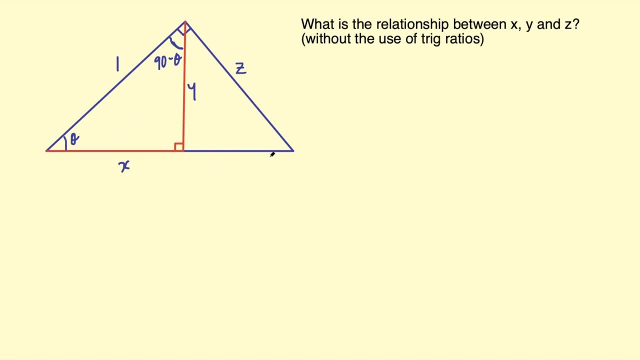 because angles are equal In a triangle. add up to 180, and also this angle over here in the blue right angle triangle will also be 90. take theta, so all of the angles in these two right angle triangles are the same. so then, therefore, we have similar triangles. So let's firstly write that down: similar triangles. 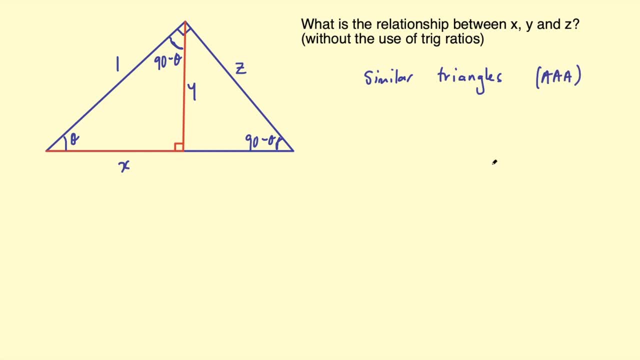 because all of the angles are the same and we abbreviate that to AAA. Then we can use the fact that sides in similar triangles are in the same ratio to find this relationship. So, looking at the legs of these two right angle triangles, the legs of the larger one are one and zed. 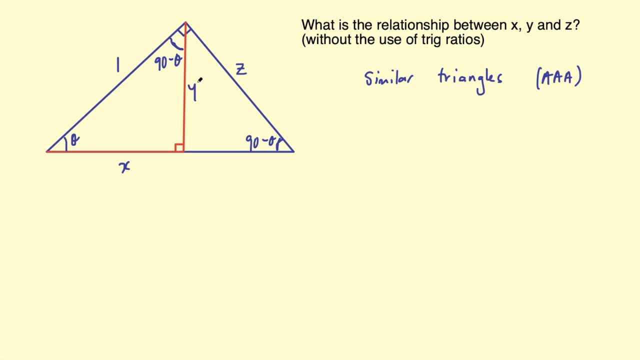 they will be in the same ratio as the legs of the smaller orange right angle triangle, x and y, and to make sure we get them in the right order we need to know which side z relates to. so this is adjacent to this angle, 90. take theta the same as y is adjacent to 90. 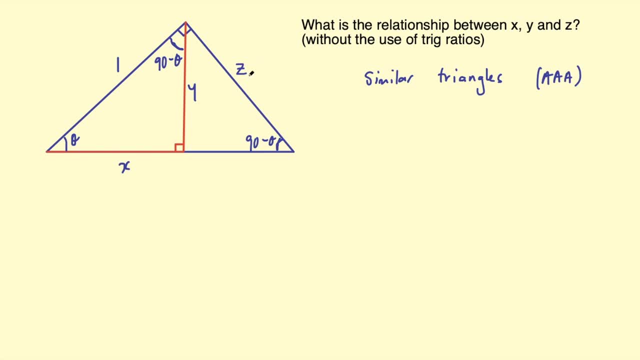 take theta in the smaller right angle triangle. so z and y will be related. so this ratio z over one will be the same as the ratio y over x. because they are similar triangles, z over one we could just write as z, so z equals y over x. so we have our relationship now: z equals y over x and this 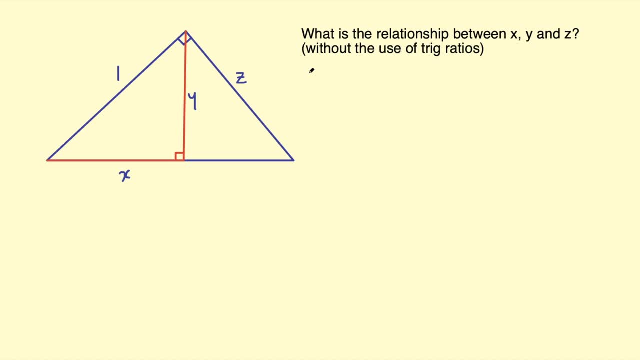 In this video I'll be talking about a geometrical understanding of the trigonometric functions and I'll briefly talk about where the names of sine, cosine and tangent come from. To show this geometrical understanding, I'll be using these two right angle triangles here, and I've written here: 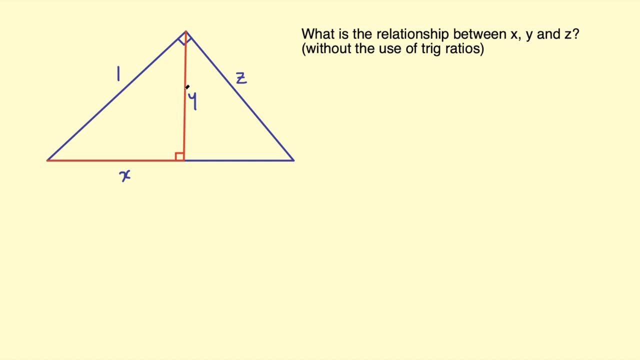 what is the relationship between x, y and z? so these lengths. and I don't want to use the trig ratios because I want to show that relationship, so I don't want to use them in my proof. So, looking at these two right angle triangles, what do you notice? Maybe pause the video here and write a few. 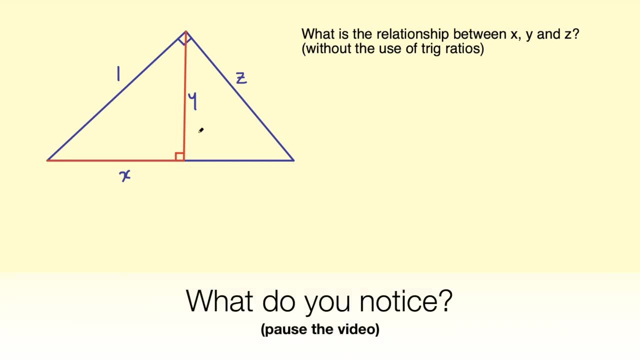 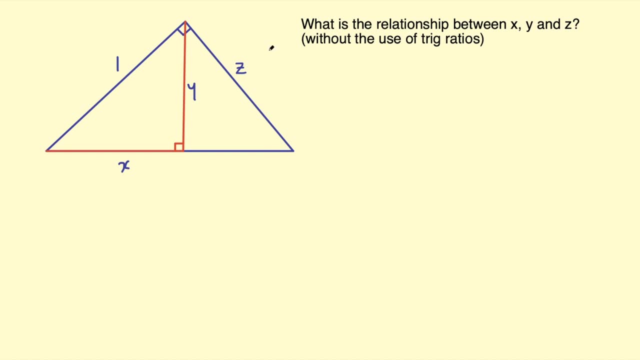 things down. The main thing is, and really the key to this relationship, is that these two right angle triangles are similar and we can show that using the angles. so if we look at this angle in here, call that theta, then this angle up here in this orange right angle triangle would be 90. take theta. 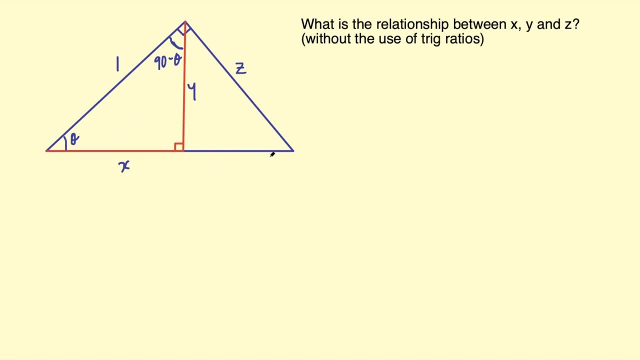 because angles are equal In a triangle. add up to 180, and also this angle over here in the blue right angle triangle will also be 90. take theta, so all of the angles in these two right angle triangles are the same. so then, therefore, we have similar triangles. So let's firstly write that down: similar triangles. 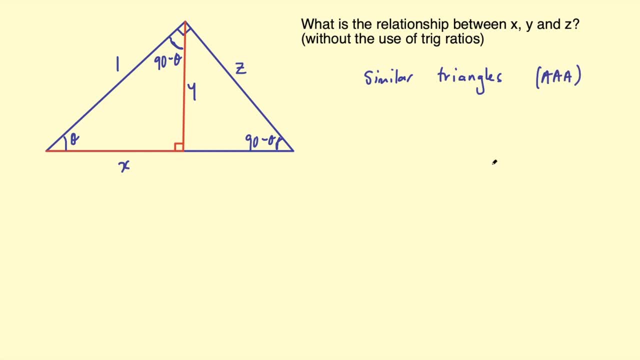 because all of the angles are the same and we abbreviate that to AAA. Then we can use the fact that sides in similar triangles are in the same ratio to find this relationship. So, looking at the legs of these two right angle triangles, the legs of the larger one are one and zed. 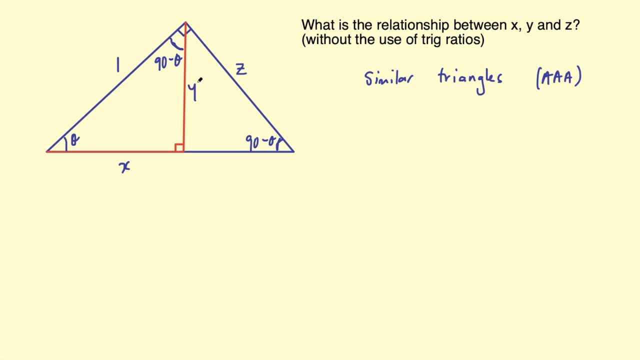 they will be in the same ratio as the legs of the smaller orange right angle triangle, x and y, and to make sure we get them in the right order we need to know which side z relates to. so this is adjacent to this angle, 90. take theta the same as y is adjacent to 90. 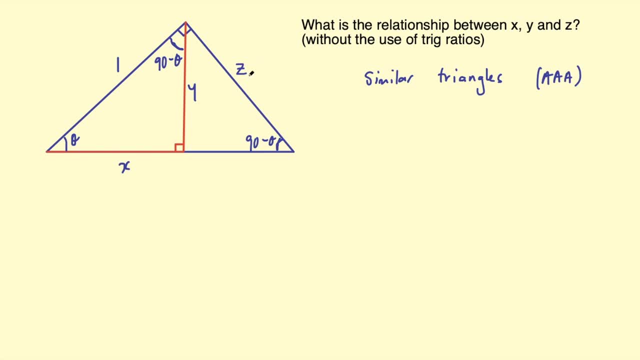 take theta in the smaller right angle triangle. so z and y will be related. so this ratio z over one will be the same as the ratio y over x. because they are similar triangles, z over one we could just write as z, so z equals y over x. so we have our relationship now: z equals y over x and this 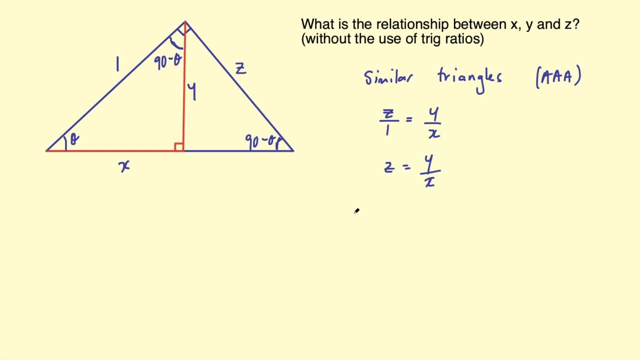 is one way to think about the trigonometric functions sine cosine and tangent. if we look at right angle triangle with a point, news of one, the this leg opposite the angle you're thinking about, so theta, in this case this side has a length of sine theta. 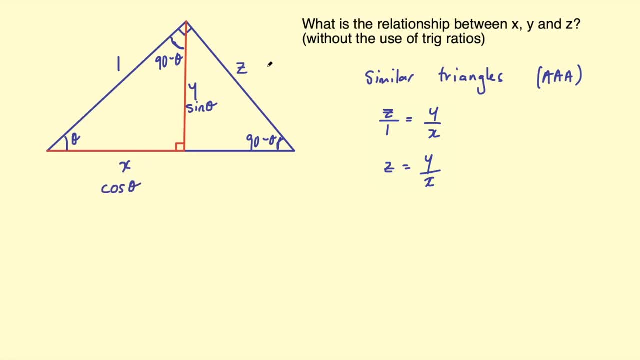 x is cosine theta and z is tan theta. and we've just shown that z equals y over x. so therefore tan theta equals sine over cosine. now you might be asking: why have i called these sine, cosine and tan theta? well, that's where the names actually come from. sine comes originally from a sanskrit word. 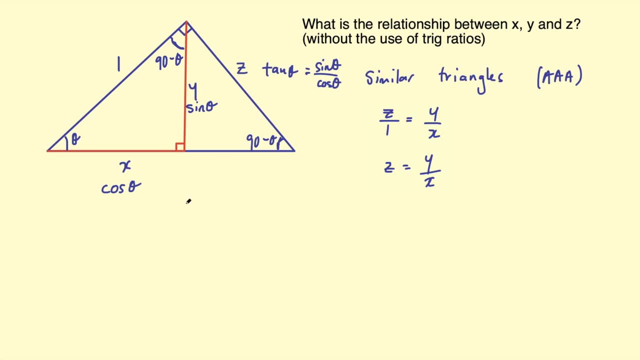 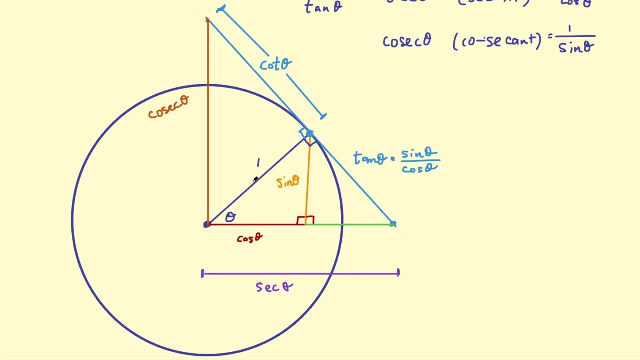 meaning half a chord. so these two right angle triangles actually relate to a unit circle. unit circle is a circle with radius one, and i'm going to pull up a diagram to show you exactly what i'm talking about. okay, here is what we call a unit circle, because it has a radius of one. 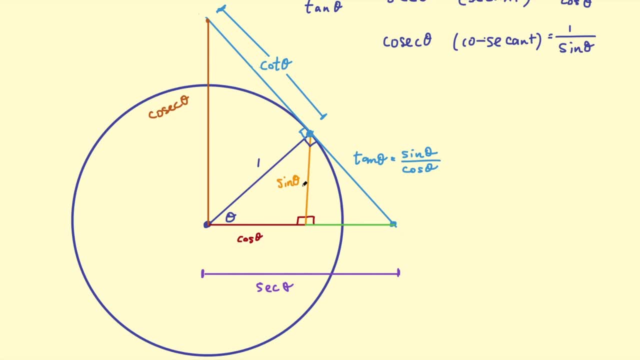 and in here are those two right angle triangles we were just working with. now there's a few other things around here. i'll get to that in a second- but i just want to focus on these two right angle triangles. this is what we originally called y. this is what we called x. 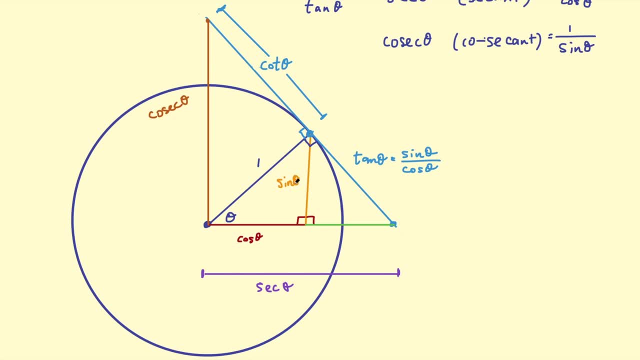 and this is what we called z here and now i've labeled them sine theta, cosine theta and tan theta. we use the unit circle because it's a way of representing every single right angle triangle with any angles within it. so as we move this radius around the circle, we create all the 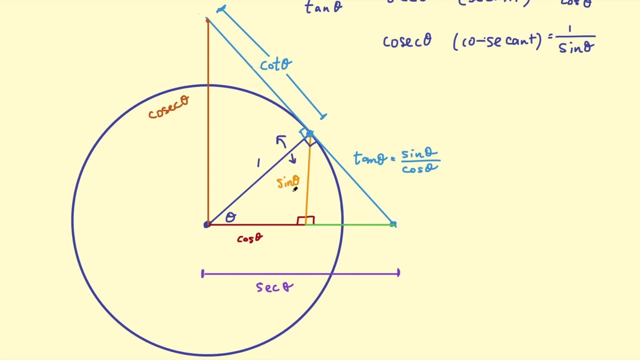 different right angle triangles and this relationship still holds. we still have sine theta, cosine theta and tan theta, equaling sine theta over cosine theta, as we just proved using theta as the angle, meaning we proved it for any angle and this is the reason it's called the. 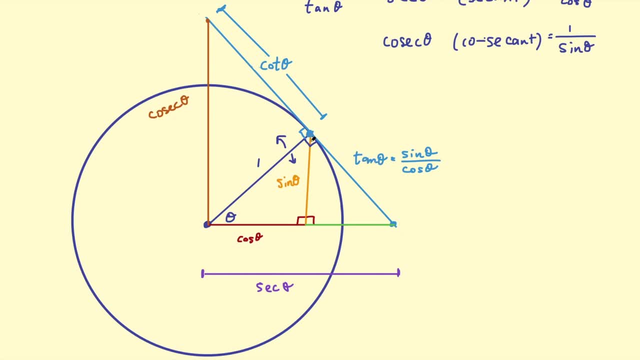 tangent, because we know that the tangent is 90 degrees to the radius of the circle. so this line, then, must be the tangent to this circle. therefore, that's where it gets its name from, and we just proved it equals sine theta over cosine theta geometrically. so that is how i 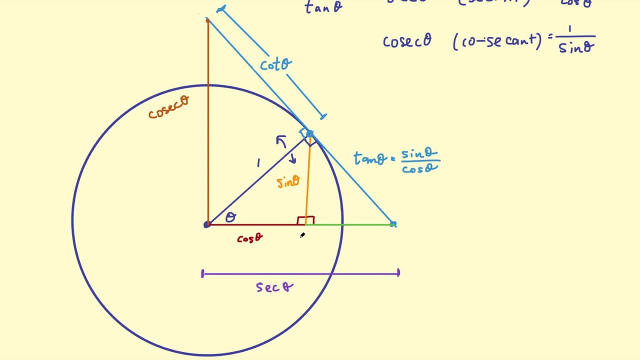 like to understand, or one of the ways i like to understand, the tangent function, because it gives it kind of a concreteness or a geometrical understanding, as opposed to the way of understanding it through ratios, etc. if you're like me and you like thinking about these. 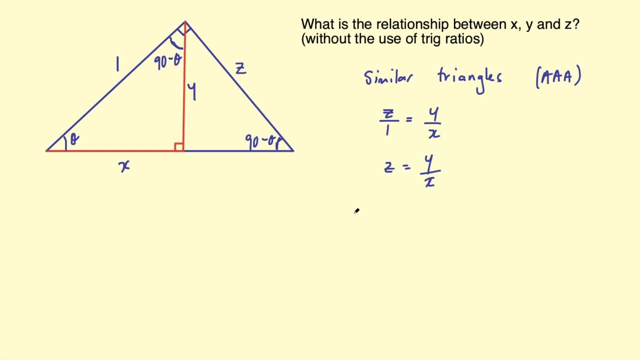 is one way to think about the trigonometric functions sine cosine and tangent. if we look at right angle triangle with a point, news of one, the this leg opposite the angle you're thinking about, so theta, in this case this side has a length of sine theta. 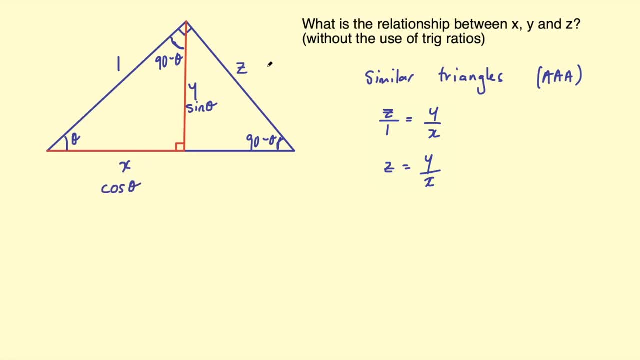 x is cosine theta and z is tan theta. and we've just shown that z equals y over x. so therefore tan theta equals sine over cosine. now you might be asking: why have i called these sine, cosine and tan theta? well, that's where the names actually come from. sine comes originally from a sanskrit word. 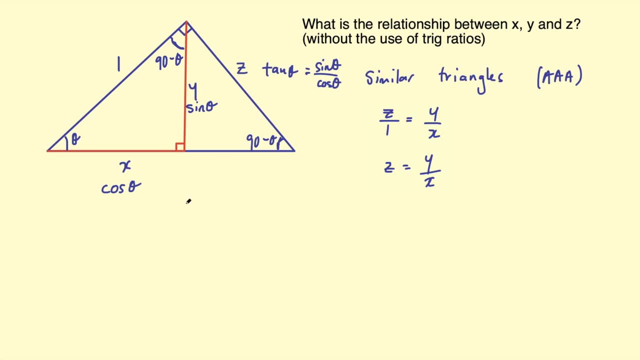 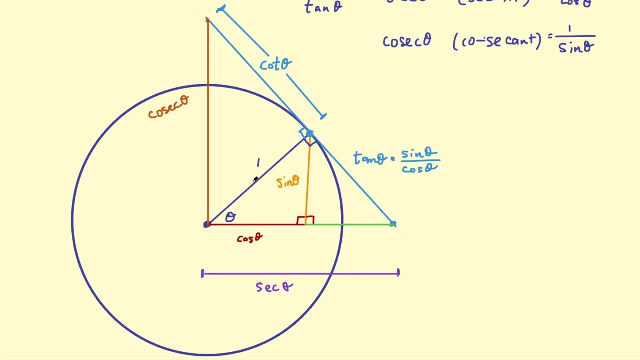 meaning half a chord. so these two right angle triangles actually relate to a unit circle. unit circle is a circle with radius one, and i'm going to pull up a diagram to show you exactly what i'm talking about. okay, here is what we call a unit circle, because it has a radius of one. 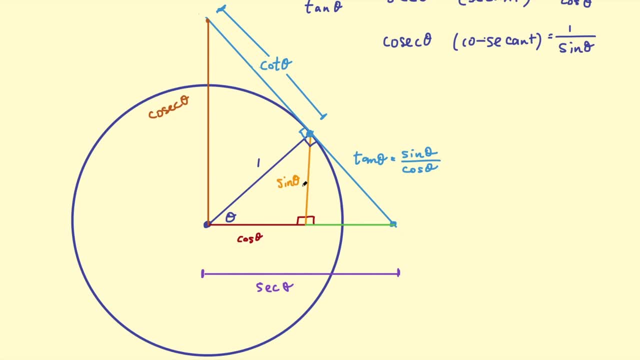 and in here are those two right angle triangles we were just working with. now there's a few other things around here. i'll get to that in a second- but i just want to focus on these two right angle triangles. this is what we originally called y, this is what we called x and this is what we called. 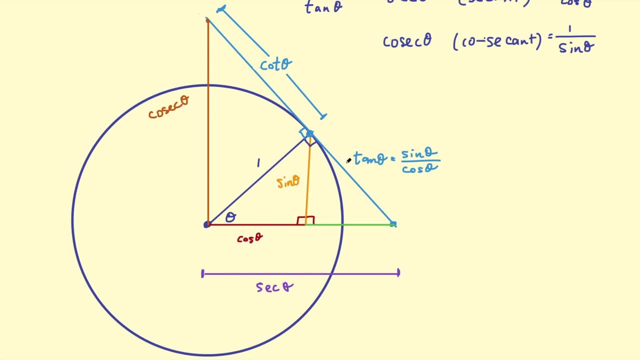 z here and now. i've labeled them sine theta, cosine theta and tan theta. We use the unit circle because it's a way of representing every single right angle triangle with any angles within it. so as we move this radius around the circle, we create all the 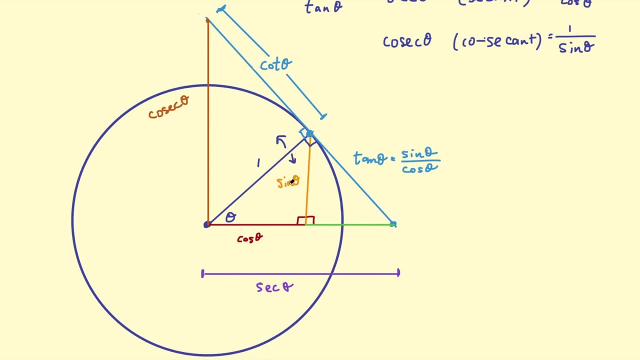 different right angle triangles and this relationship still holds. we still have sine theta, cosine theta and tan theta, equaling sine theta over cosine theta, as we just proved using theta as the angle, meaning we proved it for any angle and this is the reason it's called the. 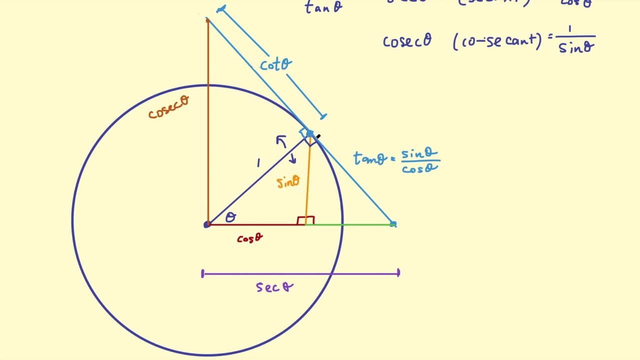 tangent, because we know that the tangent is the angle that we're going to be using, when we're going to be using the unit circle, and the tangent is 90 degrees to the radius of the circle. so this line, then, must be the tangent to this circle. therefore, that's where it gets its name from.